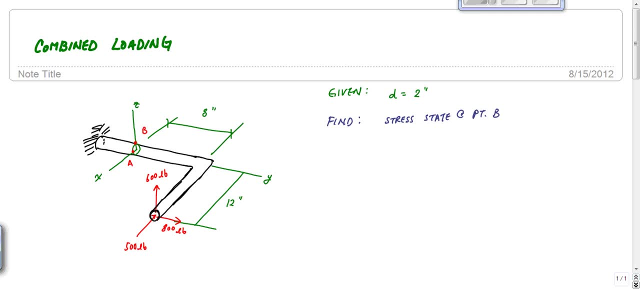 All right. so combined loading problem here. Got a rod sticking out going like that, some sort of pipe deal, And it's got some 3D XYZ coordinate system and put dotted lines right here like this for the Y axis. The diameter of this is two inches all the way through And you want to find the stress at point B. Oh, and we want to draw the different draw lines. 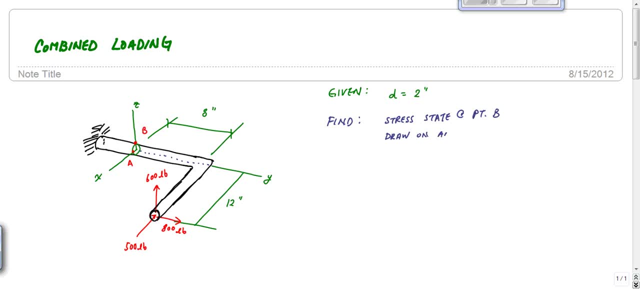 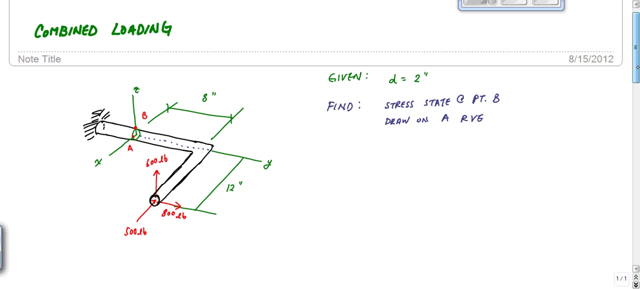 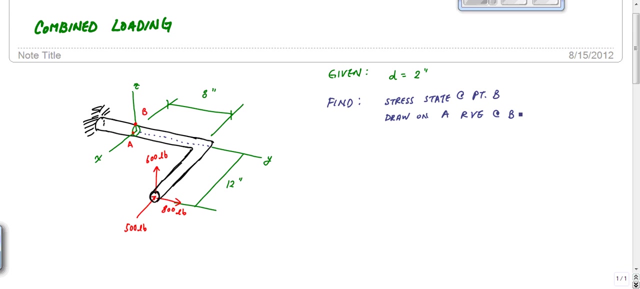 Draw on an on A RVE on a representative volume element. Okay, And so the first things first. as with anything right here, we want to find it at A, draw on a representative volume element at B, At B. So the first things first. we got to find the internal loading at location AB, which is 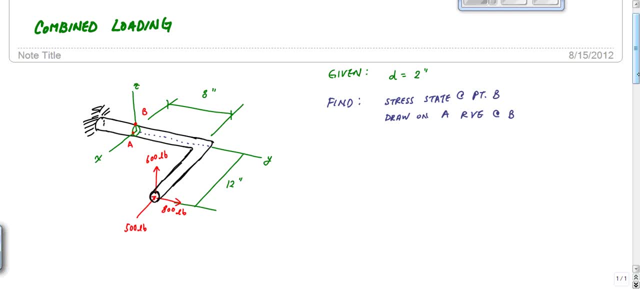 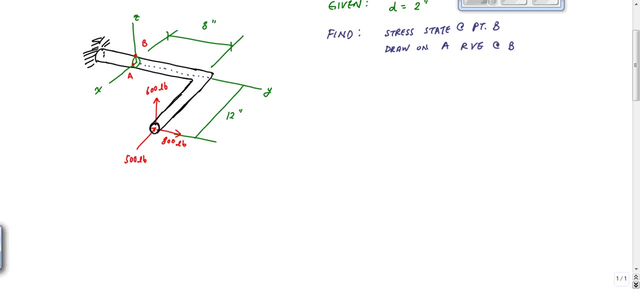 eight inches from right here, 12 inches from here, So it's not going to be too bad, But the? you know, the challenge with these 3D problems is the. the is is keeping everything straight. Okay, keeping everything straight, But this is all straight up from statics. So here one is. let's calculate one, calculate internal loading, And this is something we've done since we first. 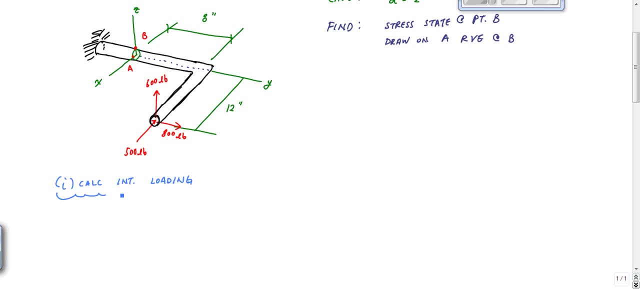 started mechanics, right It's. it's so, so fundamental to mechanics, calculating the internal loading. And if you can't do that, you realize that your problems are going to probably suffer. But here, if I, if I cut it right here at this eight inches- and let me, I'm going to draw a little bit bigger here- So if I make this cut right here and this is here, and then the rest of the pipe is coming out like: so I got a good drawing is important here. So let's. 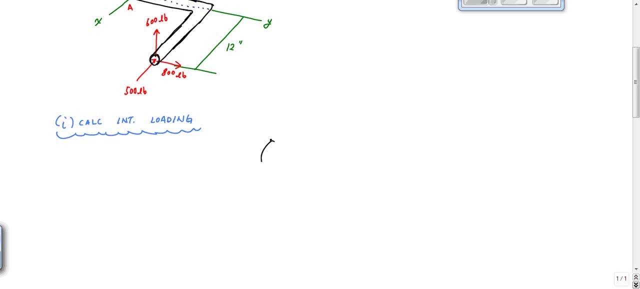 see here I will let me cut it like bam, like this here, And then the the pipe is coming out like this right here, And this is the other part of that pipe. Okay, When I add the shading, does that look like it's 3D? Not really, huh. 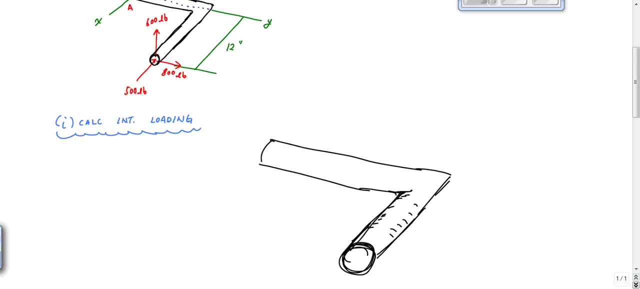 Gosh. that's why I'm not into- I'm not a graphic artist or anything- But here, this is 600 pounds, This is still 800 pounds And we have 500 going into this way. And what you want to do here is important is: is that, okay, I have this? this cut surface right here? Okay, I want to make you, want to make sure you draw the coordinate system the exact same way. So here I have. 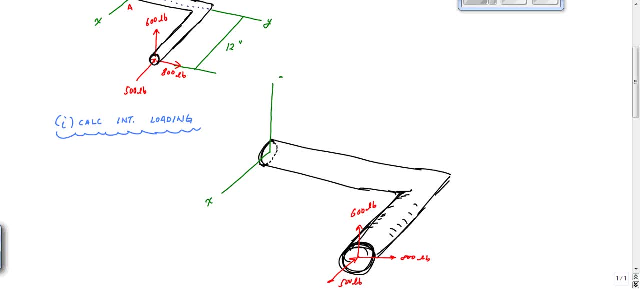 X We have. Z was going straight up And Y is coming out right here, like that. And what you want to do also is now, instead of trying to remember like positive bending, negative bending or anything like that, you just know that you have 3D, So you have moments and forces in about each axis. So here on the inside, internal loading wise, I have a sheer force. in the X, I have a. 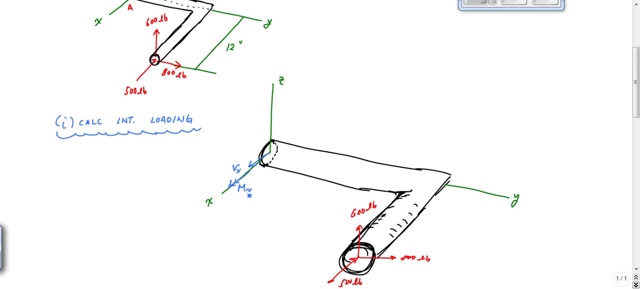 moment about the X. Okay, So this is how I'm going to draw. I have a sheer force in the Z and a moment about the Z, like this. And then I also have here I have a normal force in the Y and a moment. That's not a very good drawing: A normal force in the Y and a moment. 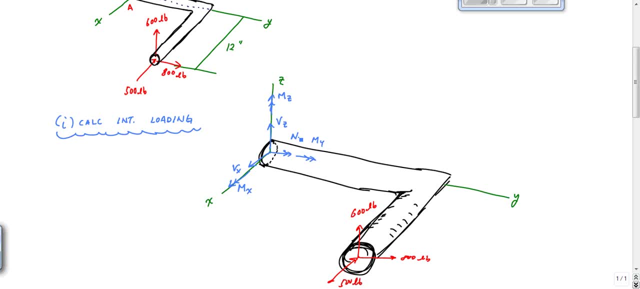 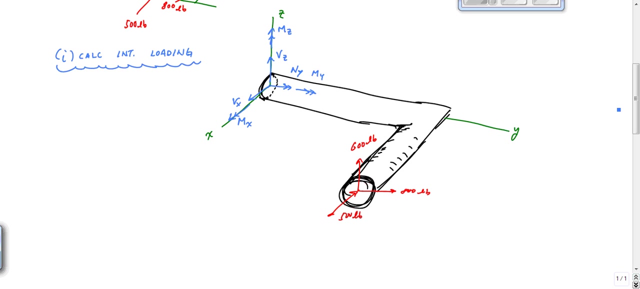 In the Y. Okay, So I'm not and I'm going to worry about what's in compression tension, what direction the stresses are going based on these arrows later. Okay, I'm not going to try to think about, I'm not going to overthink it and try to put some apply some positive sign convention to this and get confused. So here I have that right here. Now I'm going to apply equilibrium about each axis and and calculate. So I'm going to have six in this problem. here There are six equilibrium equalities. 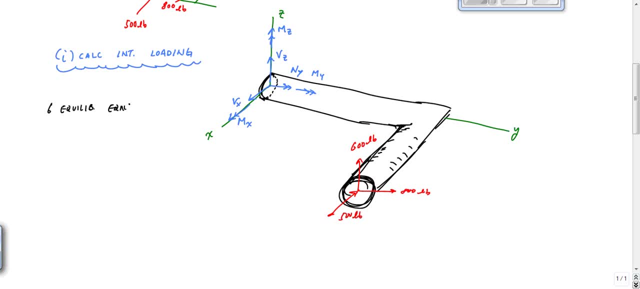 So we're going to go one at a time. So let's start with the X. Some of the forces in the X equals zero. This way is positive X. So I would have: VX minus 500 pounds equals zero. That tells me VX equals 500 pounds. Okay, Then I do some of the moments about X equal to zero And I have moments about X this way. 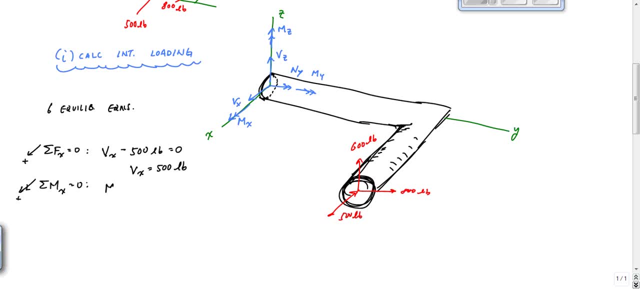 And in this case I would have MX. Let's see What induces a moment about X. Let's see: 800 pounds is on the XY plane, So no, 500 pounds is also on the XY plane, So there's no, no distance that causes rotation about the X. But I have 600 pounds times an arm of eight inches, So this distance right here was eight inches. 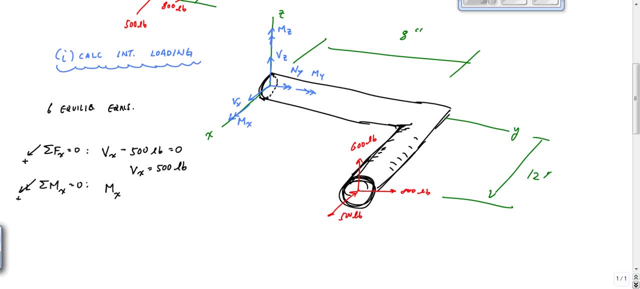 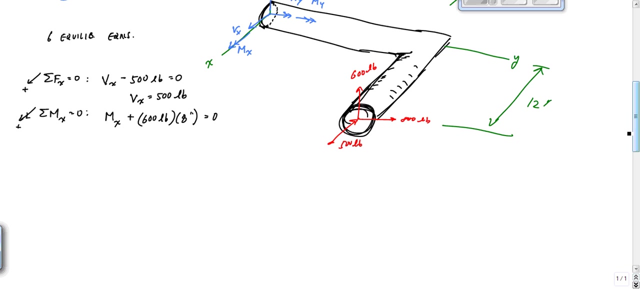 And this was 12 inches right here. So I have MX, and this induces a positive moment about X. MX is 600 pounds times eight inches, equals to zero. Yeah, Everyone okay with that. That looks okay. I can live with that Shoot, Why not? 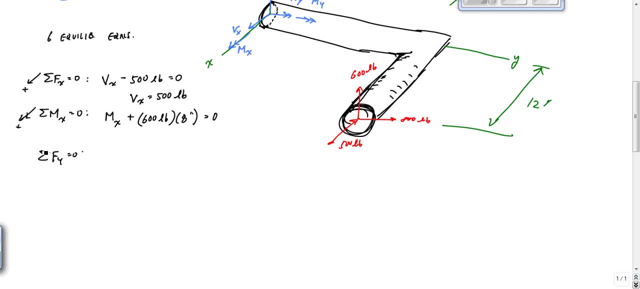 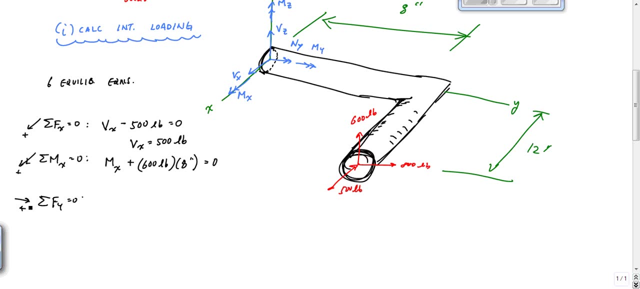 Then some of the forces in the Y equals zero. So shoot. You know, if you're watching this video right now you might want to fast forward this. But some of the forces in the Y equal to zero. This is plus. So you had NY plus 800 pounds equals zero, And that tells me NY equals minus 800 pounds. 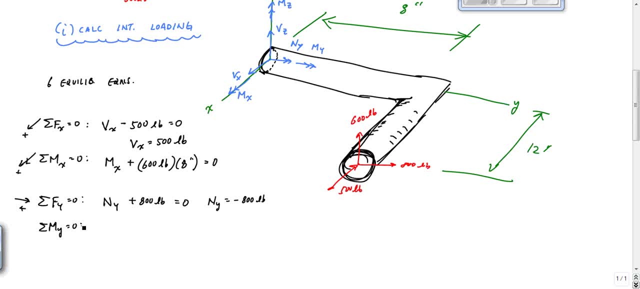 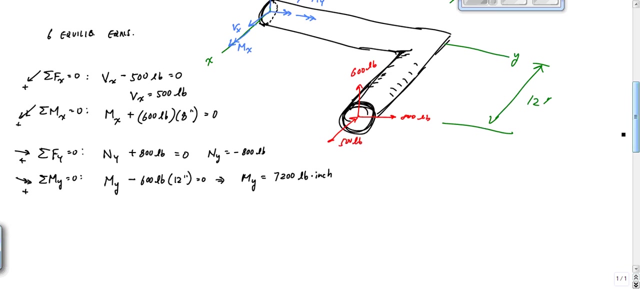 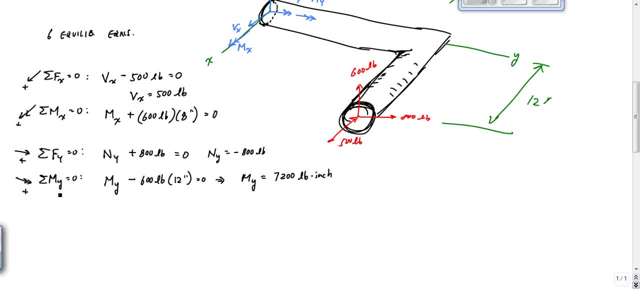 It. just it's going to be tough, Okay, It's going to be tough to do anything else. So some of the forces in the Z equal to zero, upwards this time. So here I have VZ plus 600 pounds equals zero, And that tells me VZ is minus 600 pounds. And then some of the moments about Z equal to zero, And this is positive moments about Z. So I had MZ plus 800 pounds. 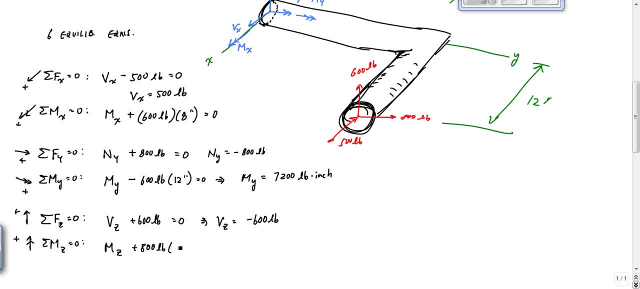 800 pounds times 12 inches And I think, oh, plus 500 pounds times eight inches. Yeah, Everyone okay with that For this 3D problem. This equals to zero, And then I would get: MZ equals some number. 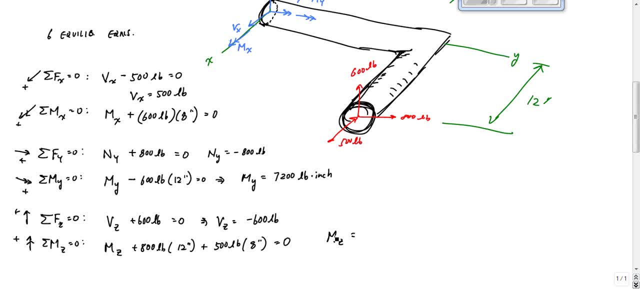 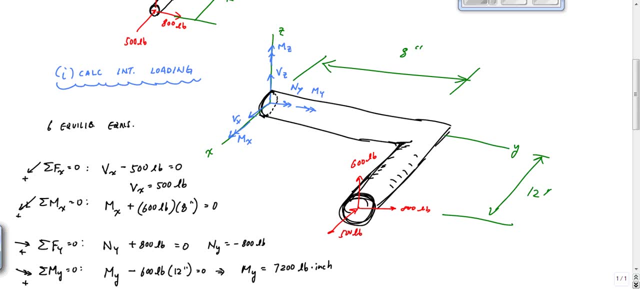 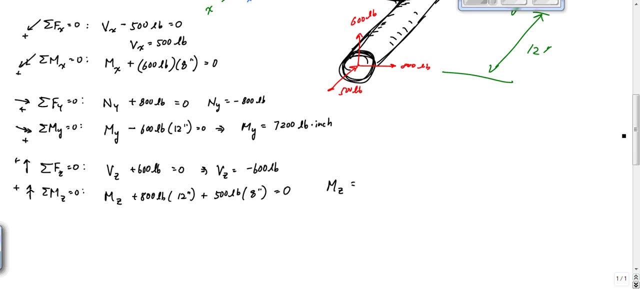 Minus No, that should be positive 500. That should be positive 500 because the yeah, it's going around, It's in the same direction as positive MZ. Okay, And same thing with the 800. Okay, So right there, And so I don't know what that 9,600 plus 4,000.. 9,600 plus 4,000.. Is that 13,600?? 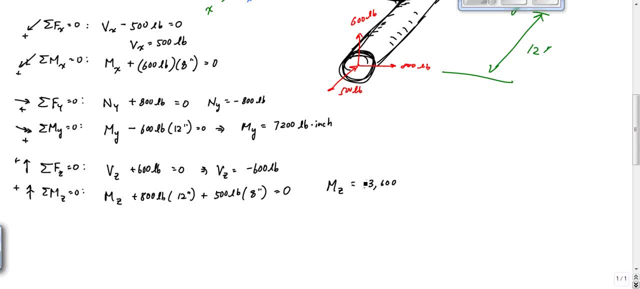 13,600 negative pound Inches. Okay, So that that's so. here are. here's my internal loading, which takes a long time, but that's that's what you have to be able to do to solve this. Oh, I need a number for this. MX is minus 4,800 pound inch, like this: 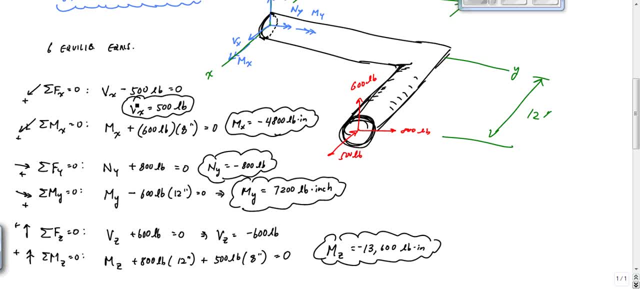 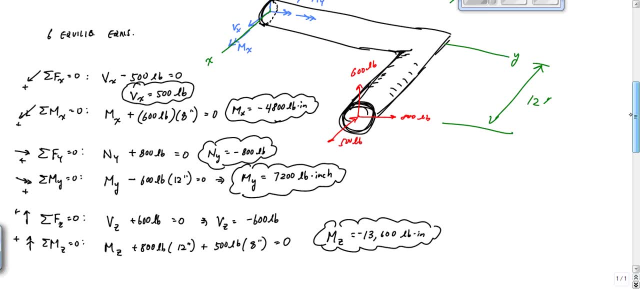 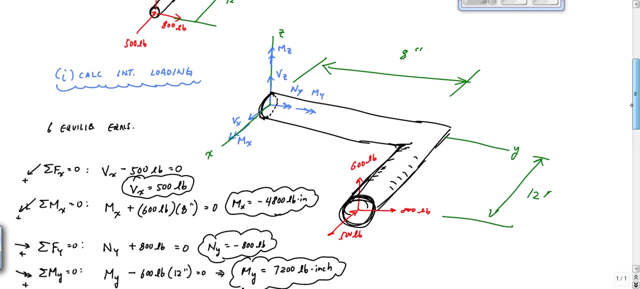 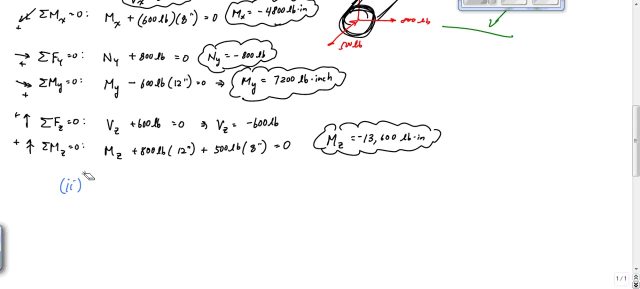 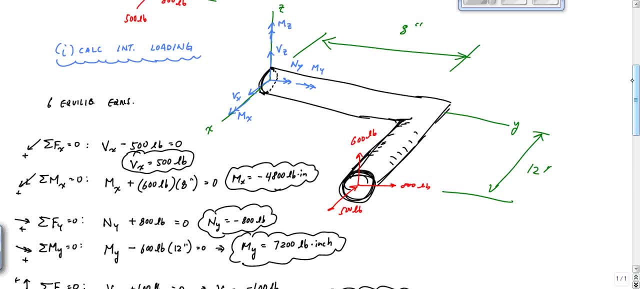 so I'm gonna draw my cross-section. I'm always gonna draw my cross-section as an observer for this problem. today, right now, I'm gonna draw my cross-section as an observer, standing over here, looking like that, okay, Looking this way at it, so that what I would see 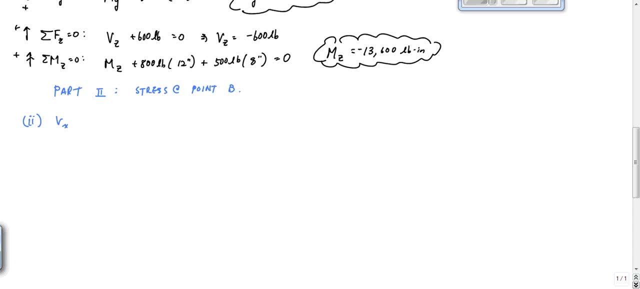 as the observer for Vx in particular, is that I would see. here's my cross-section. y would be going into the board or into the page, y will go into the page, x will go to the right and z will go upwards. okay, 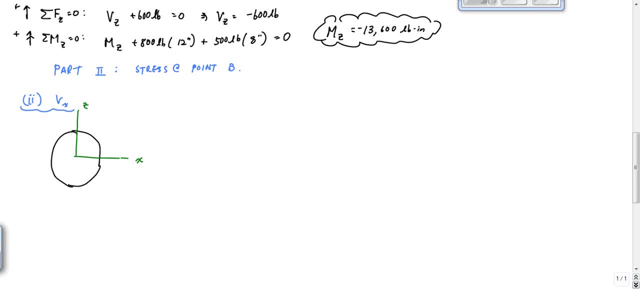 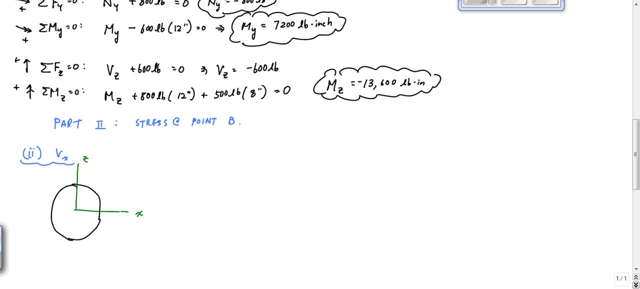 Is that okay? And Vx was: do we get a positive number for Vx or a negative number? What do we get? We got a positive number, so that means Vx goes like this: This is Vx okay. 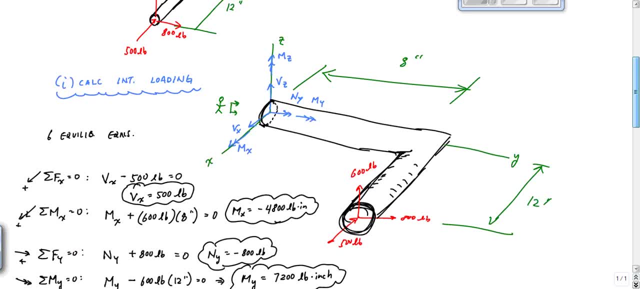 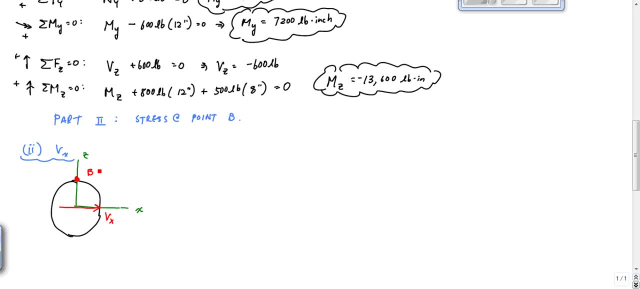 Vx is on that surface here and point A where we want to draw, or point B- excuse me, This is point B, right here. okay. So the question is: does Vx induce a stress at point B And, if so, what type of stress is it? 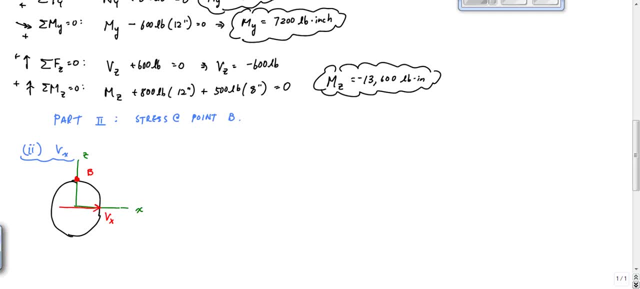 Yes and sheer are the correct answers. absolutely So here. the sheer stress at B tau B due to Vx. is Vxq over It? Okay, right here. And at point B, here Vx. we know what Vx is. 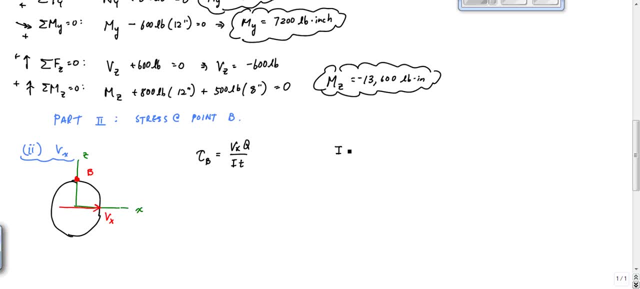 We know the direction. We also we can calculate. I. I is equal to looking on the inside cover or equation sheet. is pi R to the fourth over four? Can someone calculate that for me? Okay, T is the width of that section which, in this case, 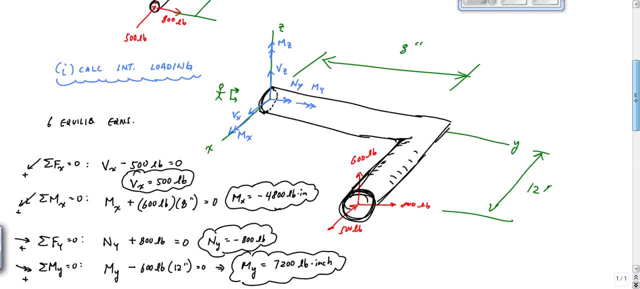 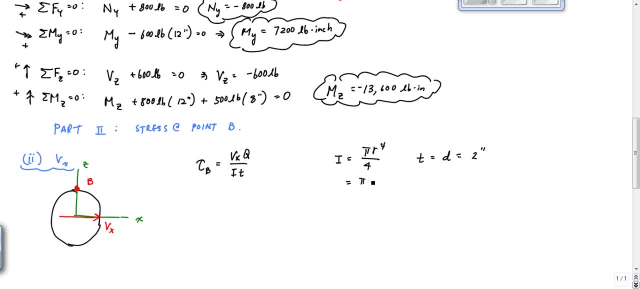 is the diameter. which is what was the diameter? Two inches, two inches In fact. oh, I don't need your help. This is pi times one inch to the fourth over four. So this is pi over four inches to the fourth. 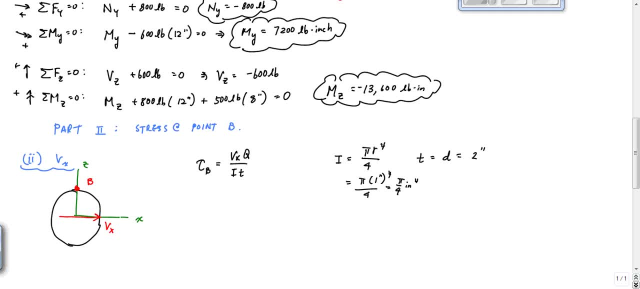 Yay, okay. And then q? q is the first moment of area of this right here, okay. So q? q is the first moment of area of this right here. So there's I, there's T, the width. 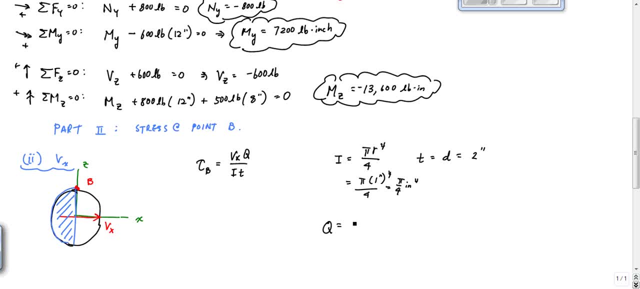 and q is equal to sum of A prime times Y bar prime, which is essentially the area of the half circle, pi one inch squared, pi R squared over two times the distance right here, the centroidal distance, You know, in this equation it would be X bar prime. 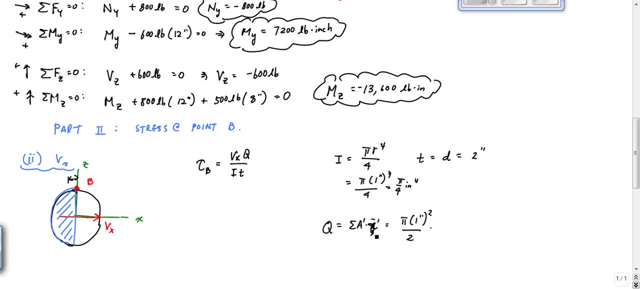 But it's okay, we're not modifying equations and stuff This distance right there to the centroid of the semicircle, which is four thirds four over three pi times one inch, Hey, hey, hey, That's two, that's pi and that is two thirds inches cubed. 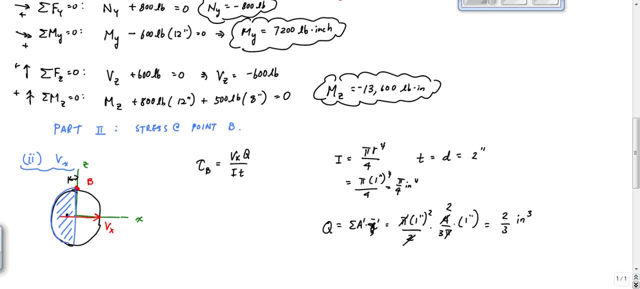 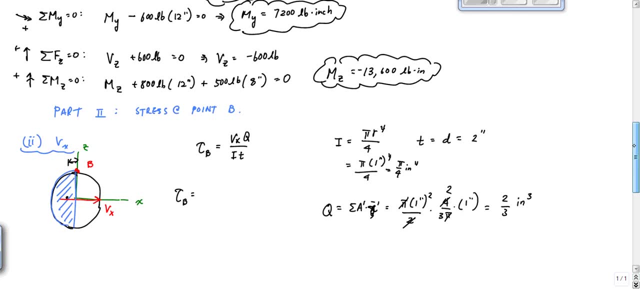 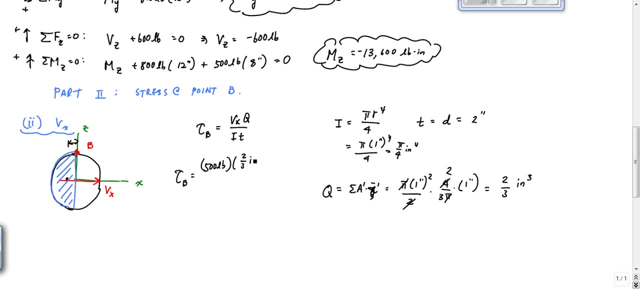 Right. Look at how nicely that works out. Wow, wow, Okay. The shear stress at B is equal to what did we say? the force was 600? No, 500 pounds times Q, which is two-thirds inches cubed, divided by I, which is pi over four inches to the fourth. 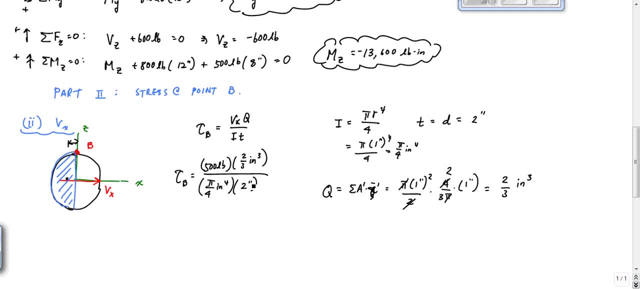 times the thickness at that location, two inches, and that gives me- I don't know what that gives me. It gives me some number in PSI. Anyone have a number Calculator? Robot Dude, it's been a long time. You guys have spent a lot of time with me today. 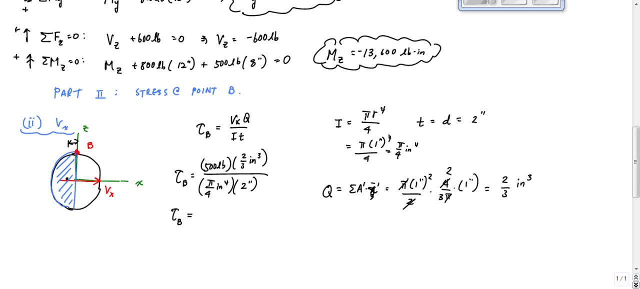 I don't know, man, I feel like two hours is a threshold with me. There's a period where I become unfunny, although I'm sure some of you don't agree with that, right? Okay, Two hundred and twelve point what? 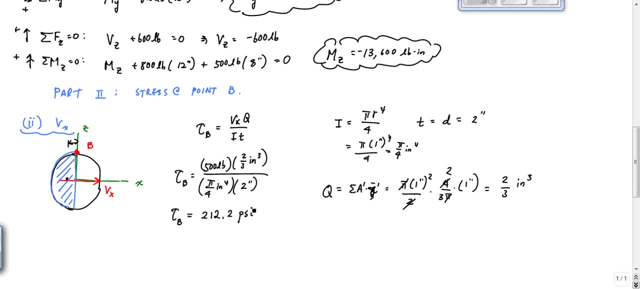 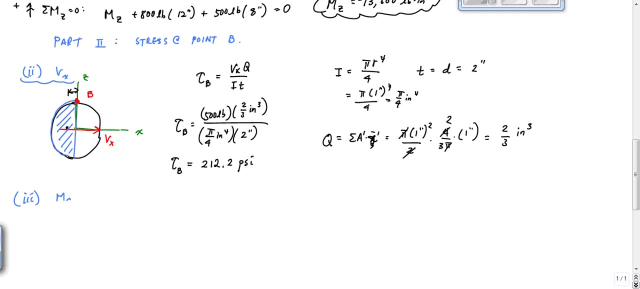 Two PSI, All right, Okay, there's one down. Let's check some more, right, Yay, Okay, So here let's go to now number three. Let's check the moment. Let's do the moment about X, okay, which we found. 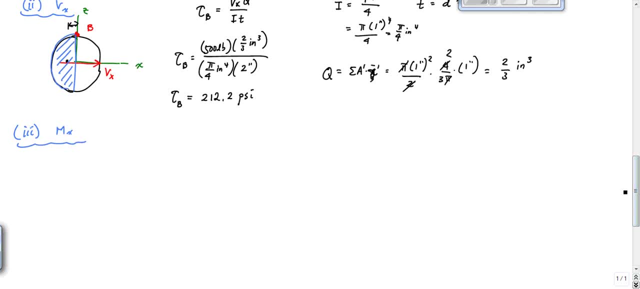 And so, again, I'm going to draw that cross-section Shoot. You know, I like to do it. I like to draw the cross-section because it helps me keep things in order. Here's X, Here's Y And here is point B. 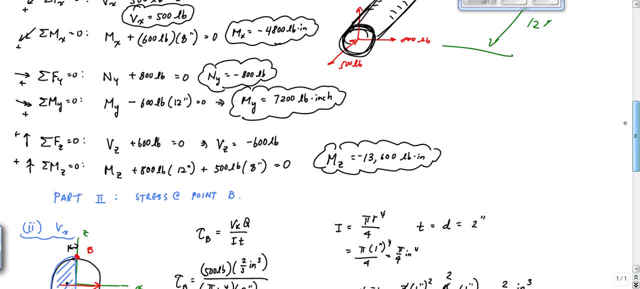 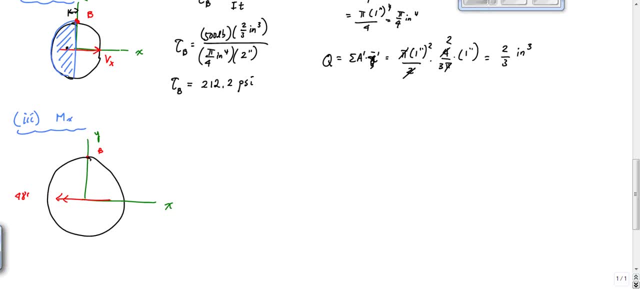 And what did we get for MX? Was it positive? It was negative: 4,800 pound-inch, which tells me that it goes this way. 4,800 pound-inch, Let's see. Okay, so does this moment about X end? 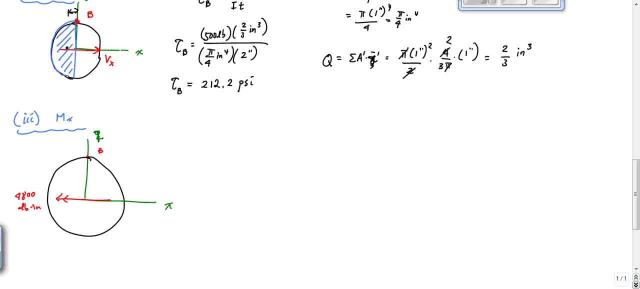 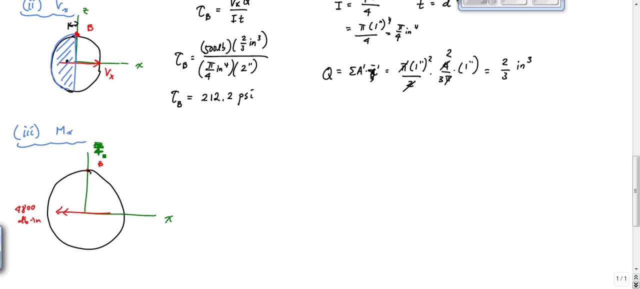 Whoa, I almost messed that up. I'm going to confuse everybody. This should be Z and Y should be into the board. okay, right there, it should be a Z. And so now does this moment- 4,800 pound-inch- induce a stress at point B? 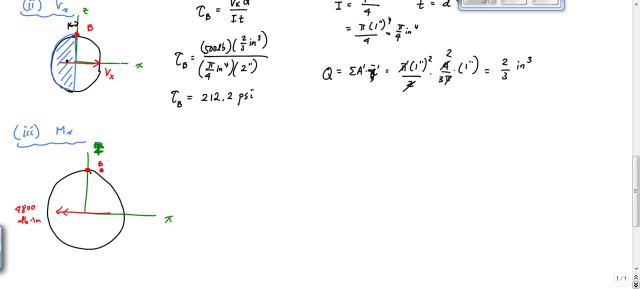 And the answer is yes, and it is normal, just like me. normal right. Normal stress at B is equal to: oh snap, you know we had this minus MY over I equation, but I don't know if that still works here. 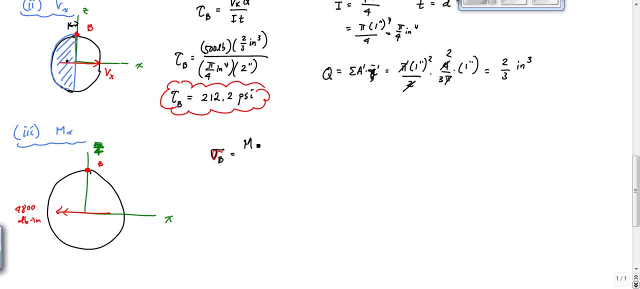 I recommend that you just calculate the magnitude of this stress- MXZ over IX, okay- And then you decide whether it's positive or negative, Or compression or tension. And what does point B experience, compression or tension, here? Compression, right, because I put my thumb in the double arrow direction. 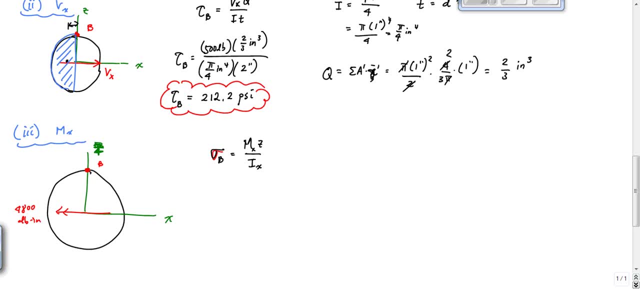 and my fingers curl to pound on B right here. So here this would just be 4,800 pound-inch. The distance Z, or the distance here to this point, right here is just the radius, or D over 2, this distance, the arm. 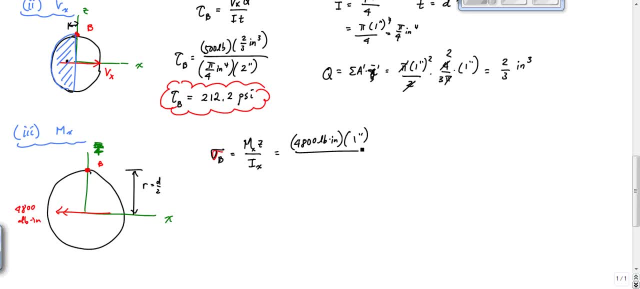 So that's just 1 inch, Yay, right. And then here, the moment of inertia which we calculated before is pi over 4, inches to the 4th. okay, The moment of inertia of any axis of a circle is still the same: pi over 4.. 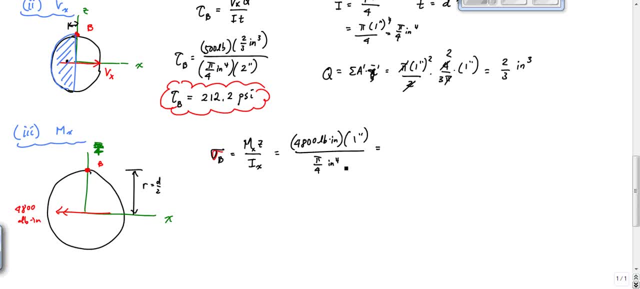 And so this is: does someone have a number for this? 6.11 KSI, 6.11 KSI And this. I will write a little note to myself saying: compression, Okay, Right here, And that was pretty easy okay. 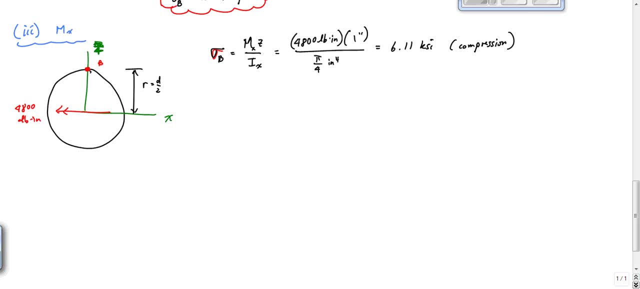 So that's pretty good. And then now let's go to number 4, which was: let's see what was the next one. Was it VY or VZ? Oh, we do. NY, NY. So let's look at NY right here. 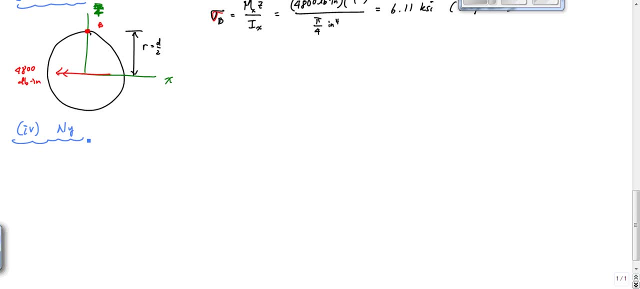 Okay, This is like a. This is a great problem. Good choice, right, We're reviewing everything, Anyway. okay, So NY, right, here was. what did we have here? NY was we had in this case. oh, I can't draw. 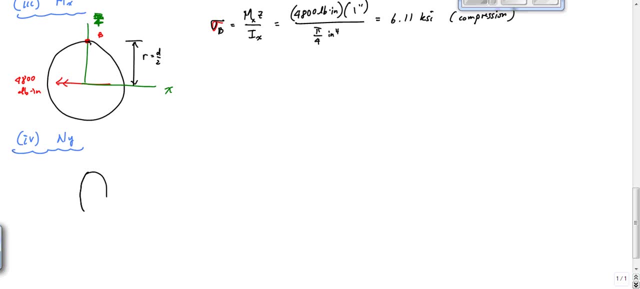 So let me draw this kind of in 3D. So here is that surface again, And here is Z, Here is X And here is the rest of my That rock, That rod right there. Okay, And that observer that we were talking about earlier is right here. 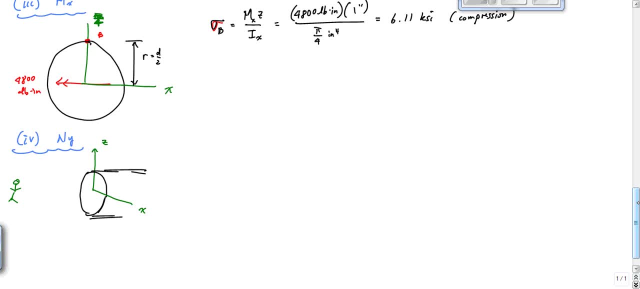 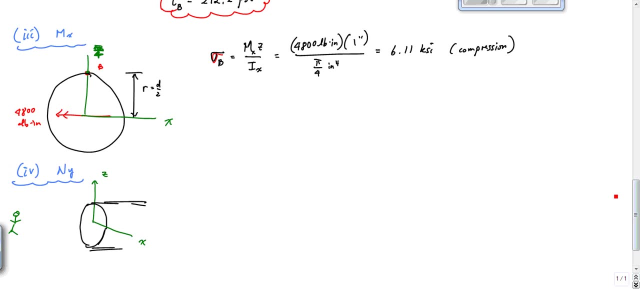 Okay, And so this NY was. what did we get? We got a negative number for NY, I believe. Okay Was minus 800 pounds, which means it is going this way: 800 pounds, Okay, And this was plus Y was this way: 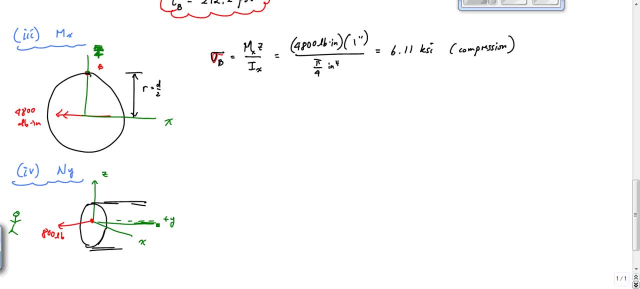 This was the Y direction. Okay, Right there And again. here is point B. right there And on the surface of point B. what is that 800 pounds doing? Is that? does that cause a stress on point B? Yes, 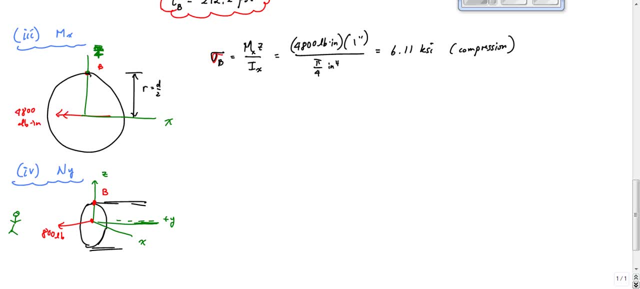 And what type of stress does that cause? Normal stress, right? My favorite kind, Sigma B, due to the 800 pounds, is just N over A And that is just going to be 800 pounds over pi R squared, pi one inch squared, which is 800 divided by pi PSI, which is- could you give it to me in KSI, this one? 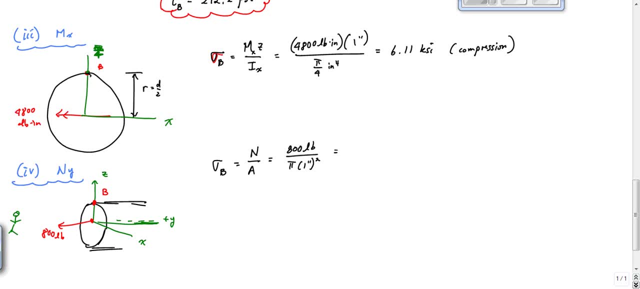 Anybody? 800 divided by pi, so 0.255.. 0.255? Yeah, 0.255 KSI. And we're not, you know. even We know that this, right here, pulling on the surface, means what? for that point B? 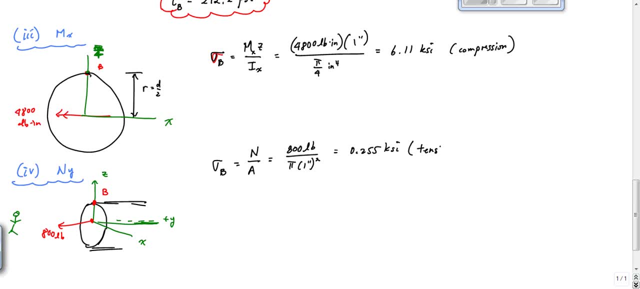 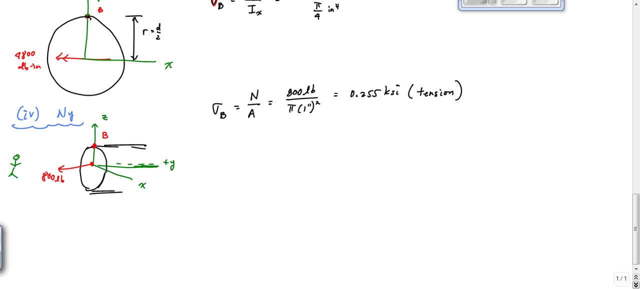 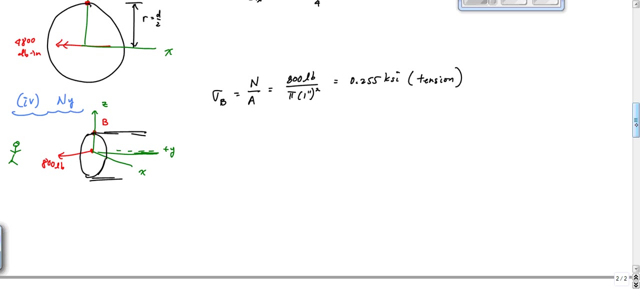 Compression or tension Tension. So we want to note that as well. Tension here: Okay, Great, Okay, Let's keep going. Now we have a moment about Y, So here let me break up a page here, Because I know that the direction of my 800 pounds 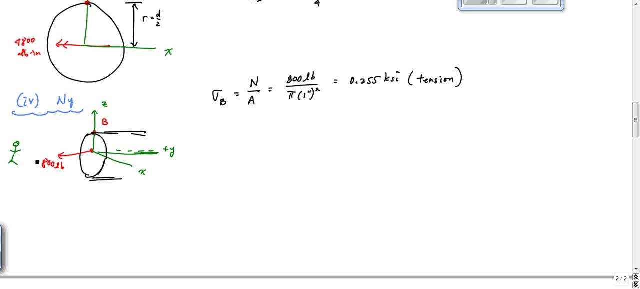 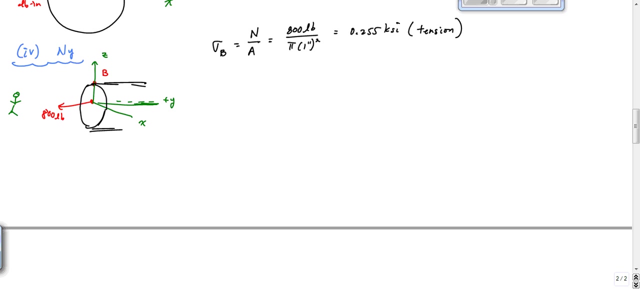 I know this is intention, because the direction of my 800 pounds is this way and it's pulling on the surface, on this area, right here, that surface. can you see my cursor? okay, all right, so right there. okay, so that 800 pounds is causing tension. now I want to look at the last part five, which is: 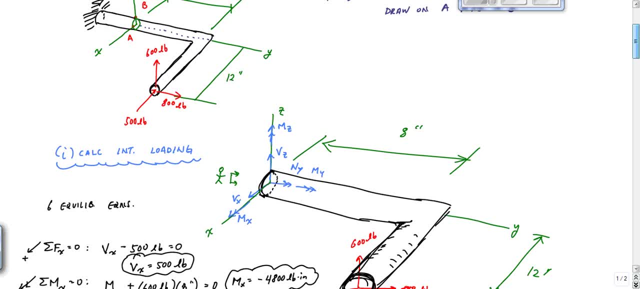 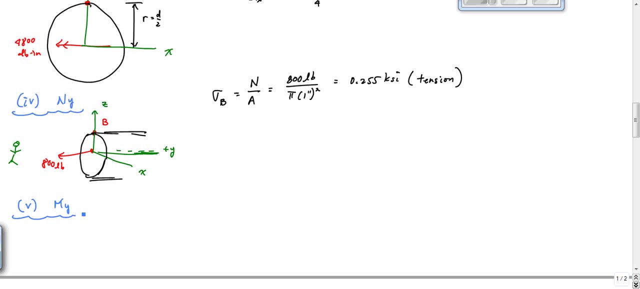 five. not, it's not the last part, I'm sorry, it's the torsion, my moments about Y and Y here and and why don't I keep the same 3d type of drawing here? so let me redraw that surface again like that, and I will. I know this is redundant and 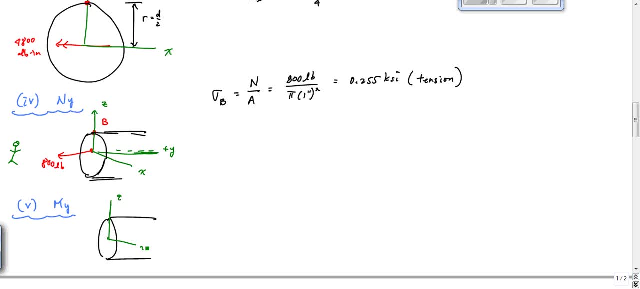 repetitive, but I just don't want there to be any confusion: X and then Y, right here, and- and I can't- I really can't- break this down for you any better than what we're doing right now. so here this X, Y, now this, do we get it?